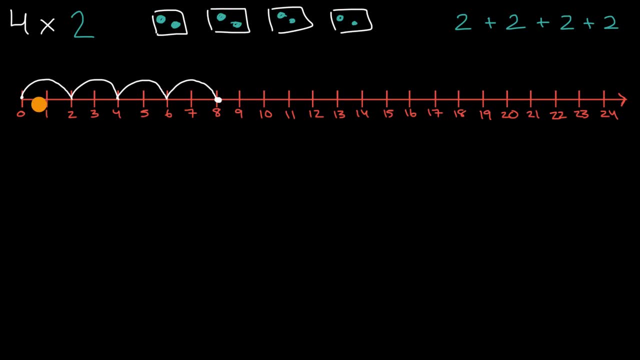 along the number line to end up at eight. We went From zero to two, four, six, eight- We just skip- counted our way to eight. So if I were to ask a similar question, actually, let me draw a little a series of hops. 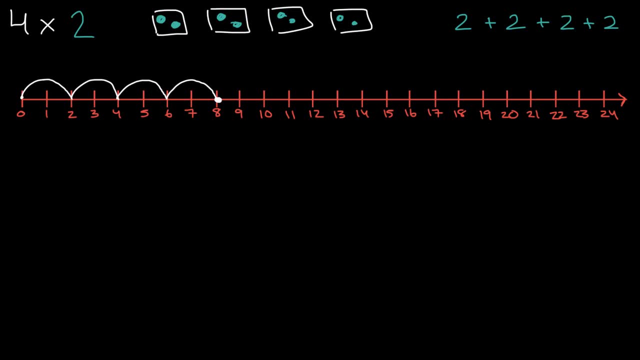 And I want you to think about it the other way. What multiplication does that represent? So let's say, I start here and then I'm going to hop like this, So I'm gonna go there and then I'm gonna go there. 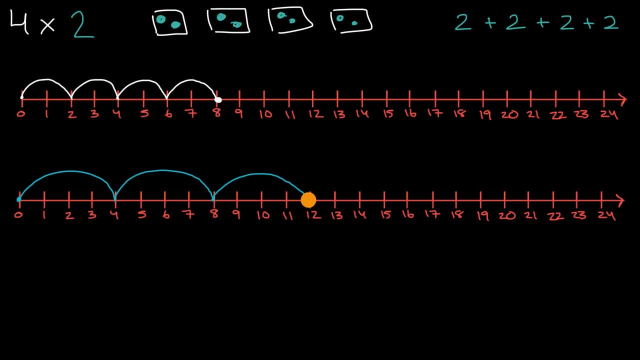 I'm taking equal jumps every time, Then I'm gonna go there, Then I'm gonna go there And then I'm going to go over there. So what would that represent if we used the same type of ideas that we just thought about? 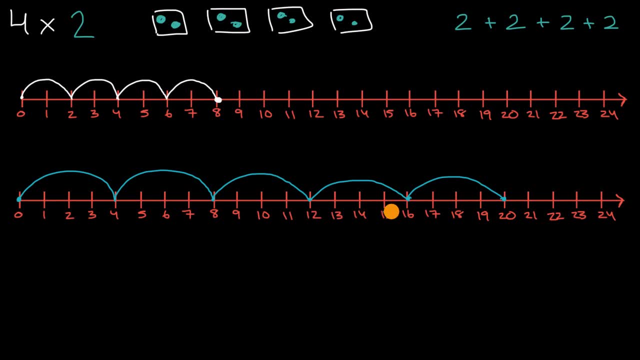 Well, I went from zero to four, eight, 12,, 16,, 20.. I'm skip counting by four, So you can imagine this is probably something times four. Now, how many hops did I take? I took one, two, three, four, five hops of four. 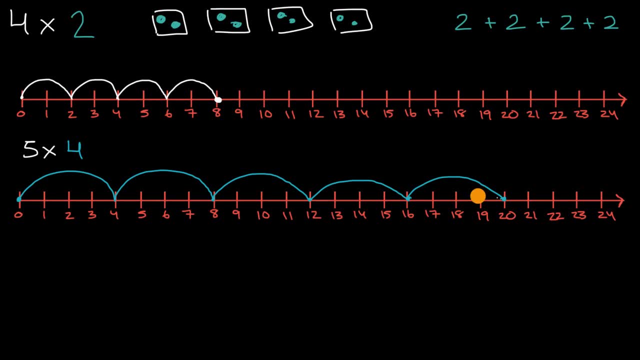 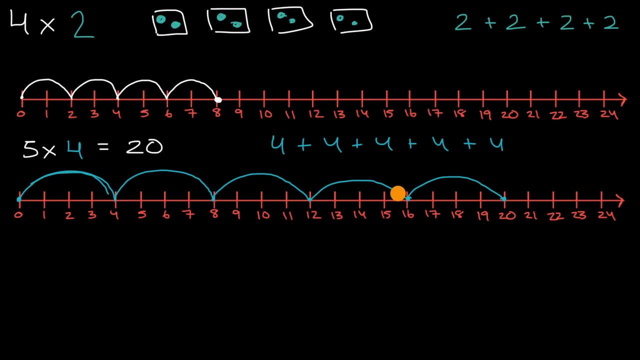 We're adding four, then another four, then another four, then another four and another four. We have five fours here. Let's do one more. So I'm gonna have a number line here And think about what's the number line. 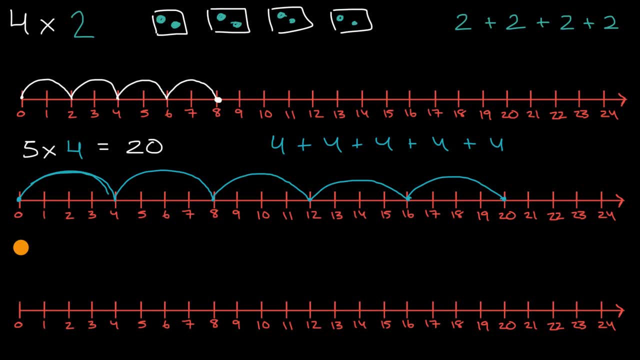 Think about what it would mean to say: do something like seven times three times three. Well, we could view that as seven hops of three, starting at zero, seven equal hops. So one, two, three, four, five, six and seven. 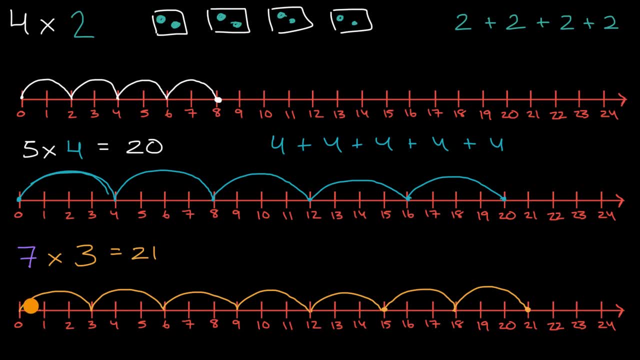 We end up at 21.. One, two, three, four, five, six and seven equal to 21.. You could also view this as we took seven threes and added them together, And you could also view it as skip counting. 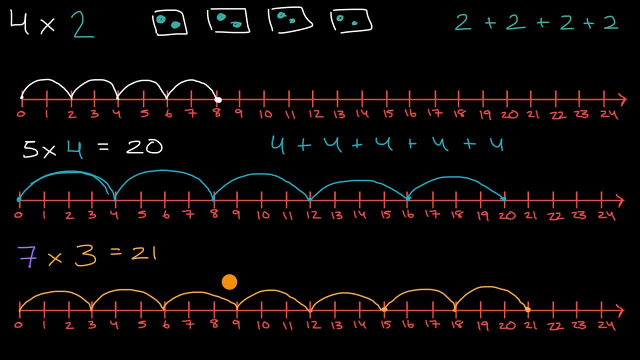 We went from zero to three, six, nine, 12,, 15,, 18, and 21.. Now, just out of interest, what if we went the other way around? What if we were to take three hops of seven?